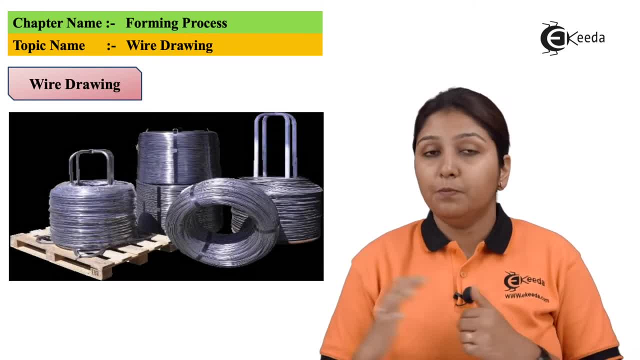 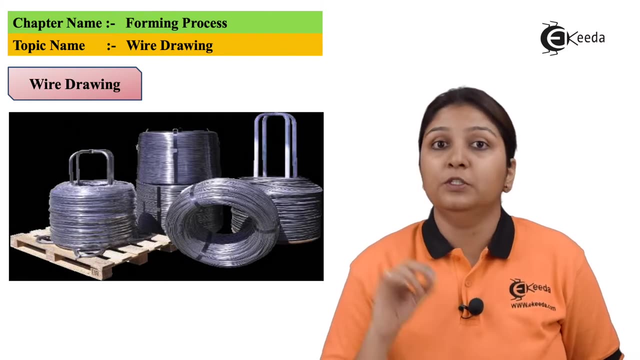 These are the basic three processes of drawing. So in this diagram you can see that there are certain wires which are WINDED. How they are made? They are made by wire drawing process, which is nothing but extrusion process- extrusion of billets- and which is further reduced to form small diameter wires. So they are. 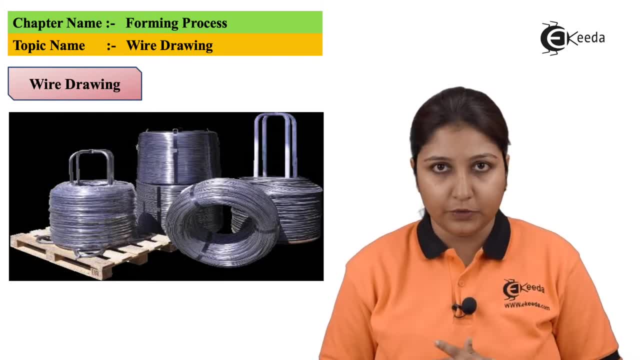 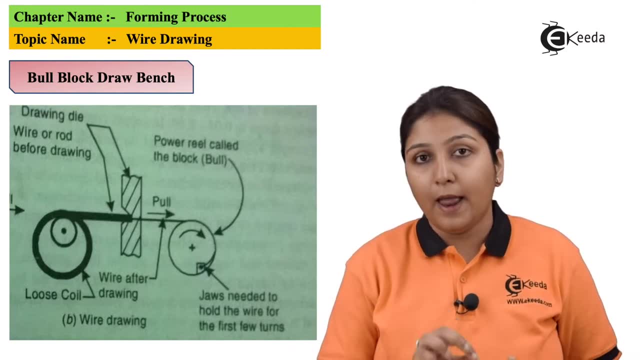 again winded and can be used in their daily purposes. Again, there is a chain block. in this diagram You can see there is a loose wire wounding and there is a small opening which has your wire to be passed and it is getting unwinded at the 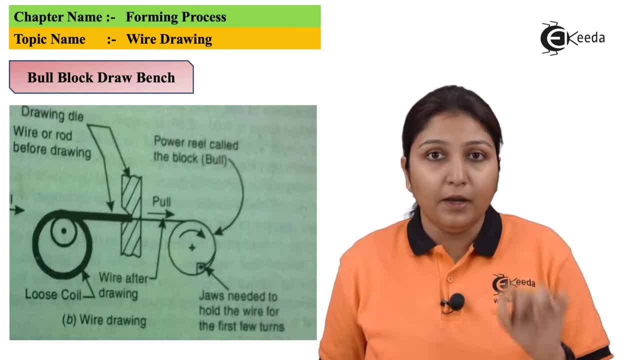 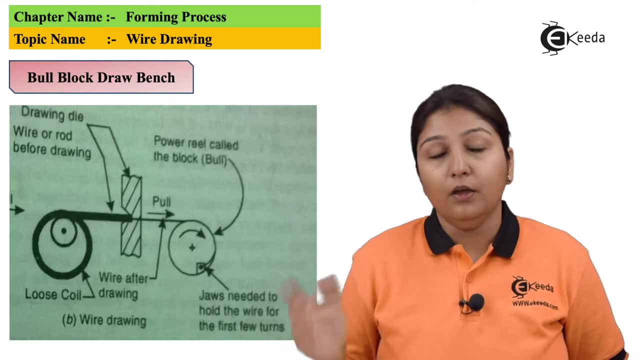 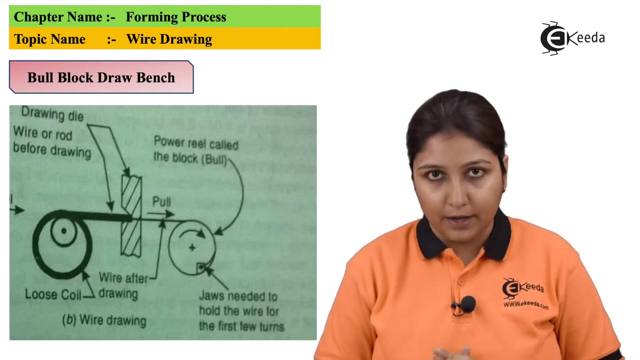 other angle. So the loose wire is your billet and it is again drawn through a small opening and getting unwinded at the other end, which is your final wire of reduced diameter. So this is known as bull blockchain diagram. In this diagram we can see a tandem wire drawing diagram. 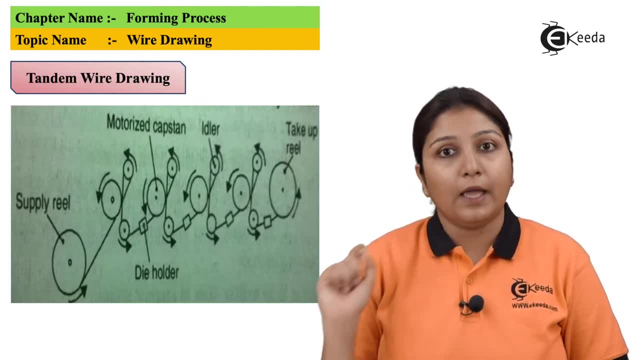 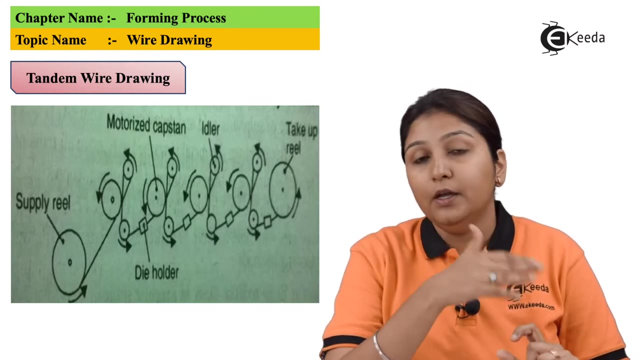 What is a tandem wire drawing diagram? Tandem wire drawing diagram is nothing but additional reduction of your wires. There are small reduction at each and every stages through that wire So that wire is big like it would be in the form of billet. It would be reducing again and again and 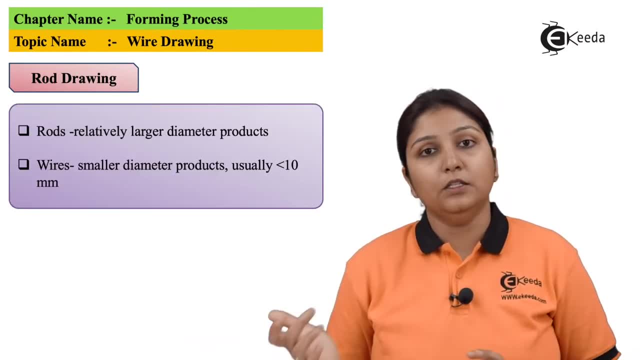 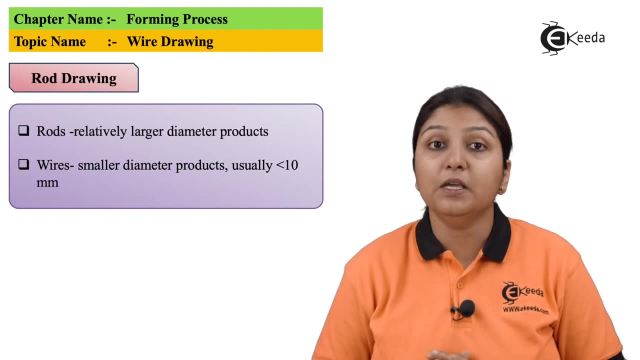 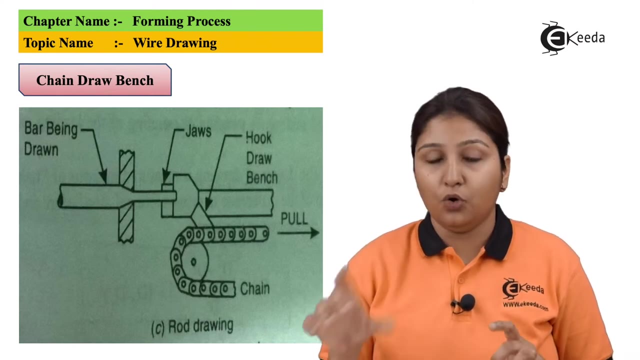 finally the final shape is being made. So by this process you can make rod as well as you can make wires of a very less diameter. So these two products can be easily made. In this diagram you can see there is a bar which is getting out from a small opening. There is a jaw or a hook which is holding it, and again it is. 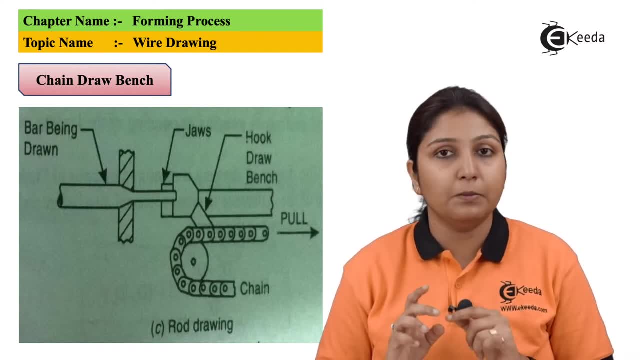 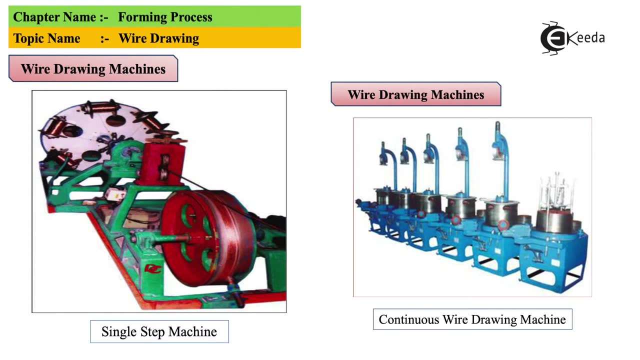 passing through a chain type structure. that's why the name is chain bench. So these are two diagrams of two kind of wire drawing machine. One is single step wire drawing machine. Second is continuous wire drawing machine. So in single step single wire can be made and in a single 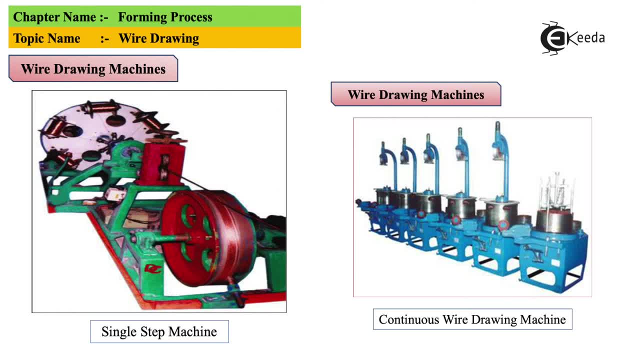 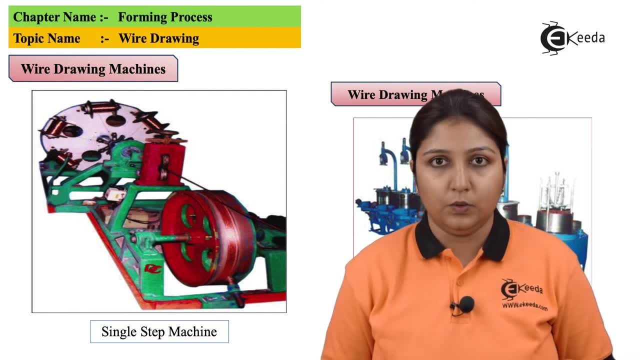 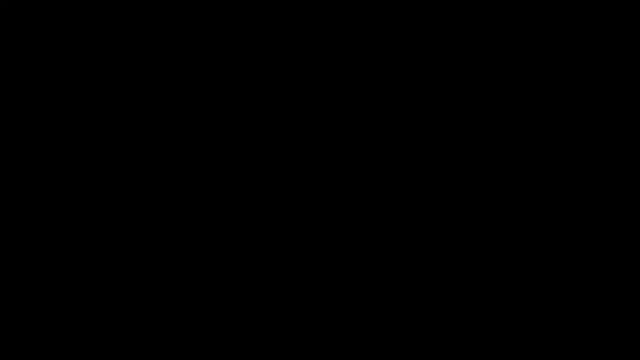 and in continuous wire drawing machine. your wire drawing process is continuous and large amount of coiling can be done through that wires. thank you for watching this video. stay tuned with ikeda and do subscribe our channel, ikeda you.